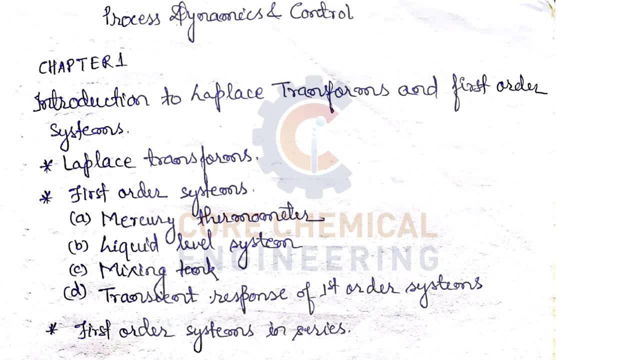 within 12 to 13 tutorials. okay, so first one. so introduction to laplace transform and first order system. so these are the topics that i'm going to cover first: laplace transfer, laplace transforms- what are all these and what is the importance of laplace transforms. then, after that, first order, 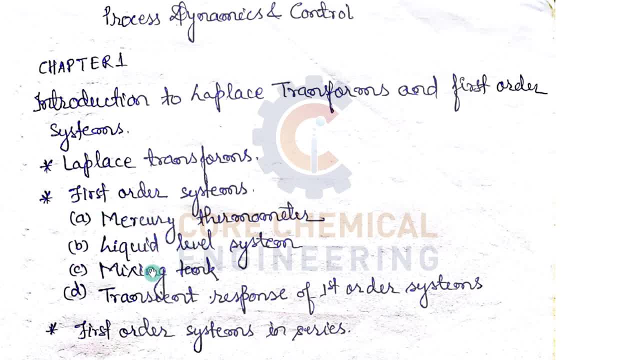 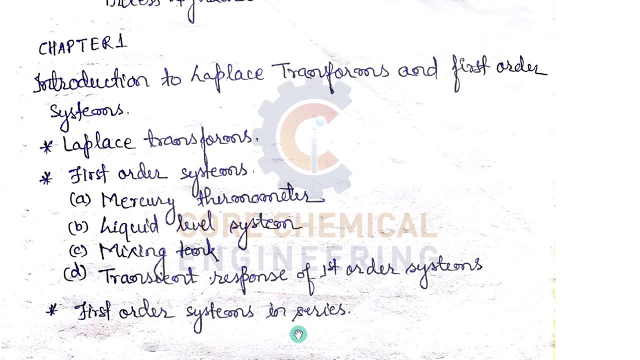 system, in that we'll discuss these four topics: mercury, thermometer, liquid level systems, mixing tank, transit response of the first system and after that we'll discuss about first order systems in series, like interacting system and non non-interacting systems. so these all will discuss in the chapter one. then after that comes the chapter number two: closed loop, linear control. 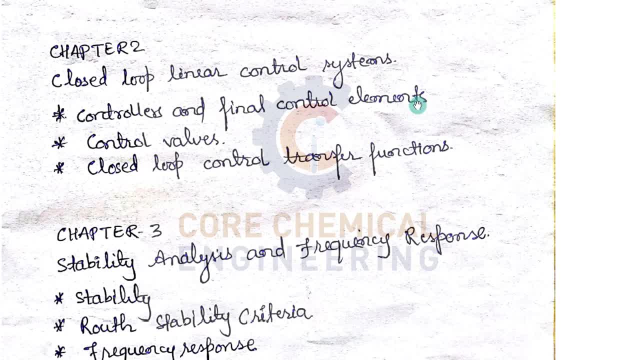 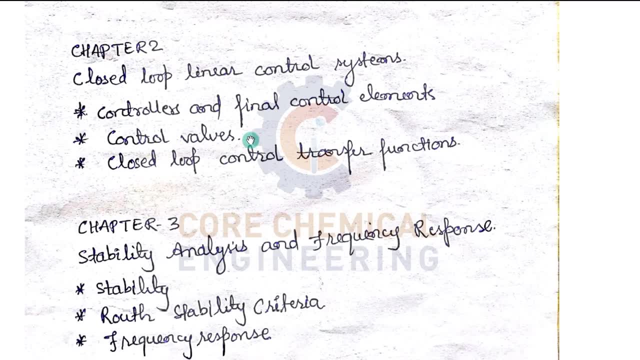 system in that we'll discuss about controls and final control element. what are these, then, control valves? what are the control valves? what in that? uh, what different types of actions of control valves, like a fail to open, fail to close air, fail to open air flow to close air, fail to lock, all these things? 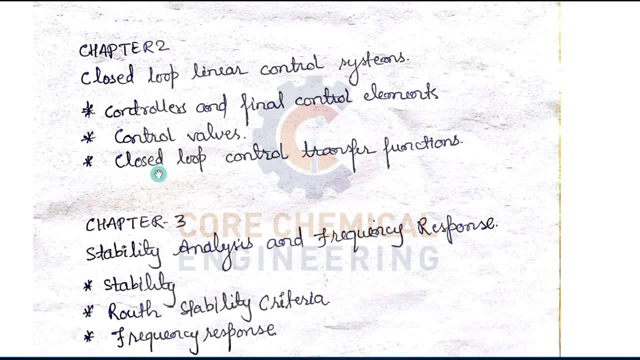 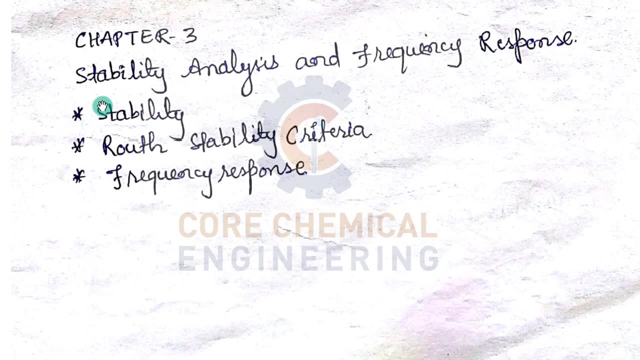 we'll discuss in this tutorial. now, the next topic that we'll cover in this chapter is closed loop control transfer function. okay, feed forward, feed backward control loop, close loop control system- all those things we'll discuss now. in the chapter three we'll discuss about stability analysis and frequency response. so in that we'll discuss stability of the system. 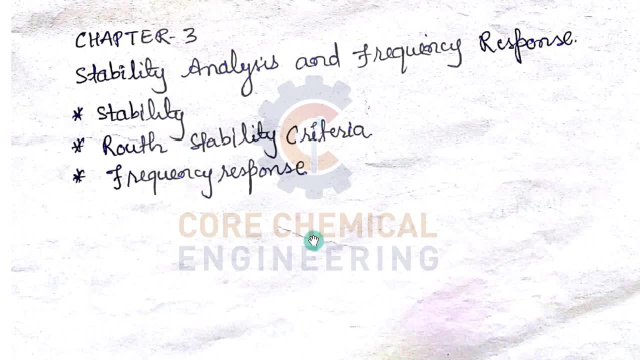 route stability criteria and the frequency response. so, apart from this, after covering all this, i'll try to explain the practical applications of this chapter, that is, that are being used in the industry, okay, how all these are related in any industry, and then after that i'll try to cover 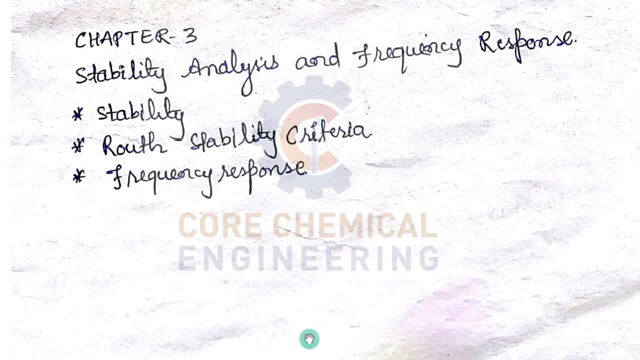 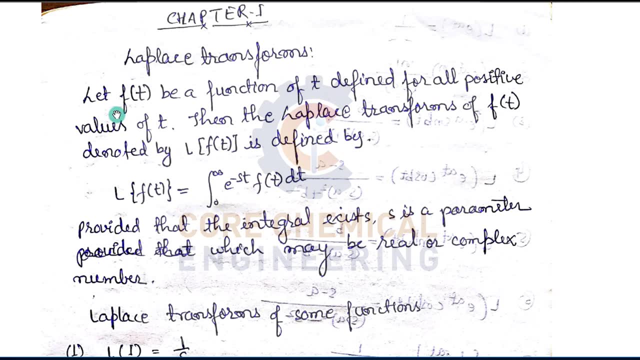 some numerical problems based on the gate exam. so let's discuss chapter first: laplace transforms. okay, so laplace transform of any function, f of t. okay, so you can see it here. let f of t be a function of t defined for all positive values of t. then the laplace transforms of f of t denoted by: 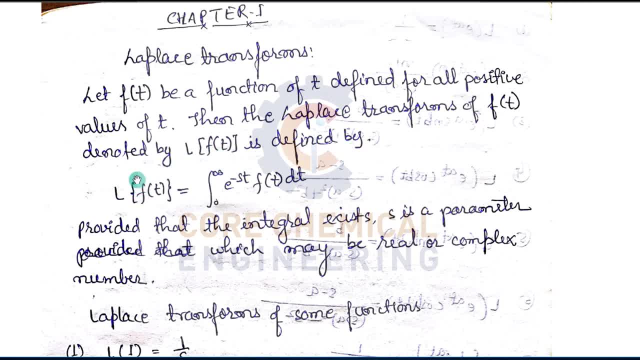 l, f of t is defined by: if you are going to take laplace, transform of f of t is equal to integration of zero to infinity. e, e raised to the power minus h, t into f of t, dt. so if you take the integration of integration of, 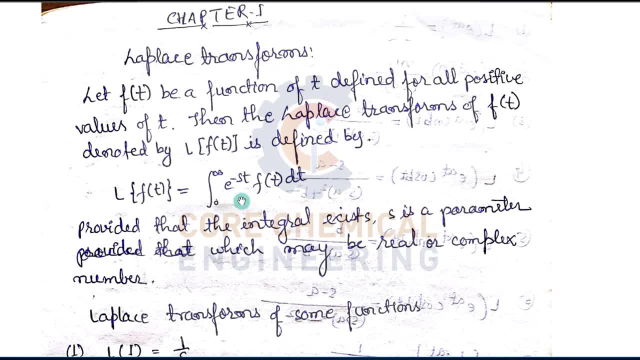 an integration of f of t into e, raised to power minus h t, zero to infinity with respect to the dt, then we'll get get the laplace transform of function f of t. now, the condition product here is the product that the integral exists. s is a parameter which may be real or complex number. 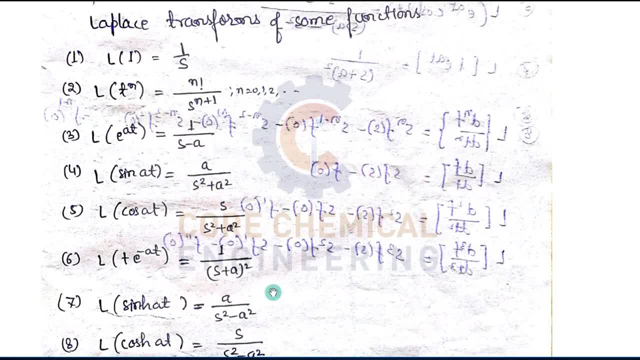 that doesn't matter now. here are the some examples of laplace transform of some functions. these are the you know the basic uh, laplace trans, basic uh formula that you must remember before you enter into the subject, like if you want to study the process dynamics control subject. these are the very basics, uh, you know, laplace transform. 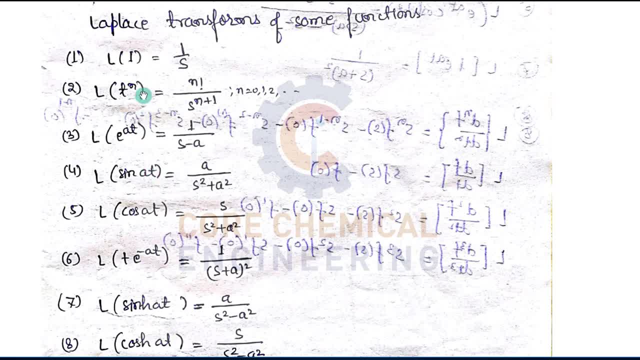 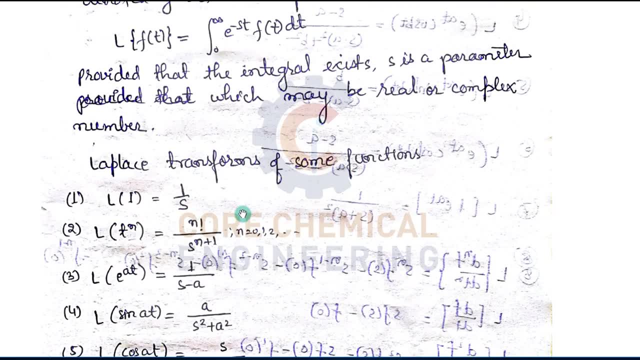 some functions that you must remember on the fingertip. so here i have written those. you just remember, and mathematically you can prove all this by using this formula. okay, so i have not derived here, i have written this formula. you just note it down and remember. first, l of 1 is 1 by s l of t raised to the power n is n factorial divided by s raised to power n plus one, where n can be equal to plus n and t cross n equal to n times s value. let's illustrate this as like this: so so, first let's see all the formulas that we will learn comfortable. so this is complete. the components of this is to be darn, so you can. 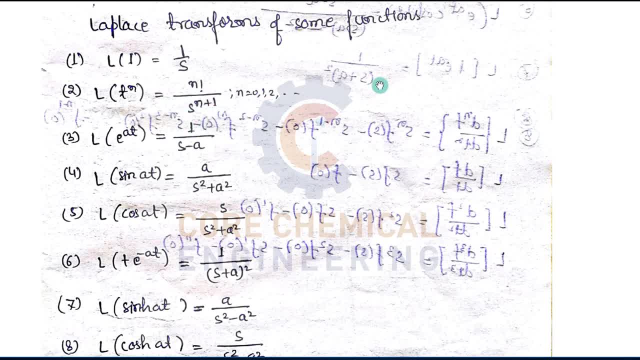 n factorial. factorial divided by s raised to power, n plus 1, where n can be 0, 1, 2 or any number, then l of e at is equal to 1 upon s minus a. l of sine 80 is equal to a upon s square minus s square plus. 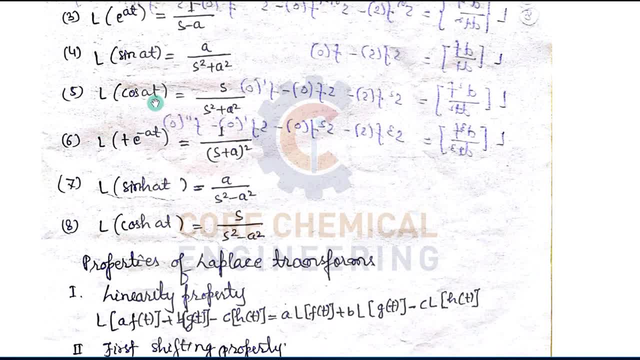 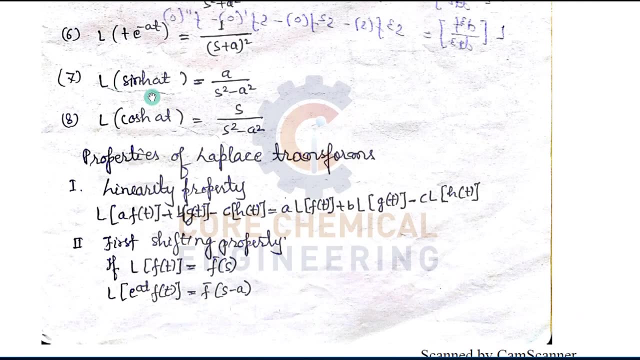 a square, then l of cos 80 is equal to s divided by a square plus a square. and then l of t into e raised, raised to power minus 80, is equal to 1 divided by s plus a square. then, seventh number, l sine h of 80- this is the hyperbolic function- is equal to a divided by s square minus a square. 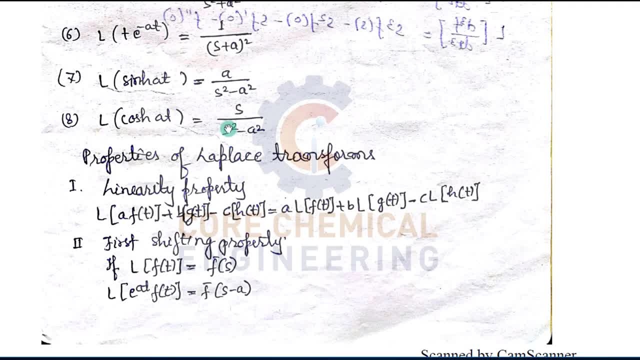 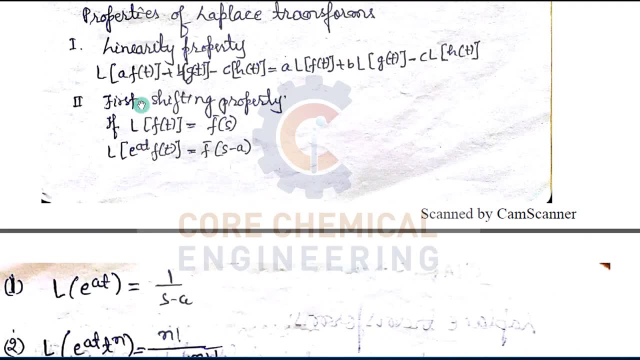 l of cos of 80 is equal to s divided by s square minus a square. so these are the laplace transform of the function that you must remember now, please, please do remember, uh the pro, some properties of laptop laplace transform also. so first property is linearity property. so if you are going to 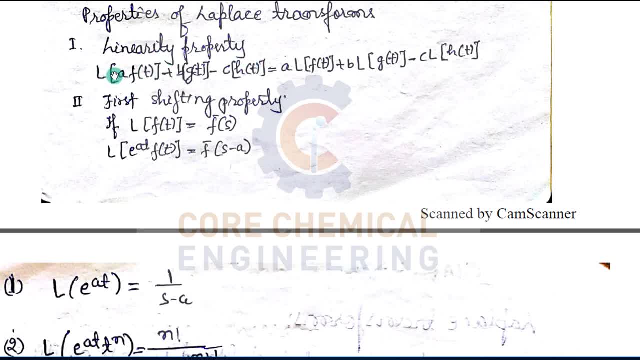 laplace transform of this complete system, uh l of a, f of t plus b, g of t minus c, h of t, is equal to. if you are, then what you can do. if, like i, you are supposed to take the laplace transform of this entire function, then if there is addition or 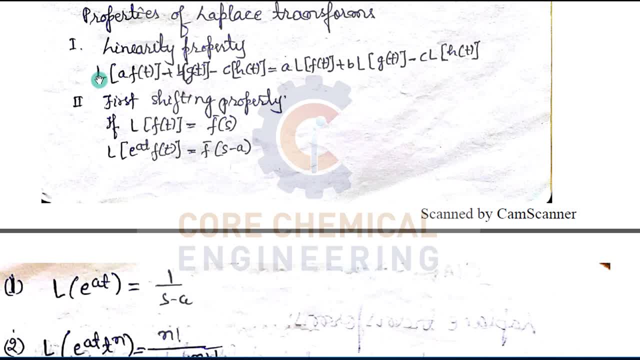 subtraction symbol is there in between. then you can take the uh laplace transfer of individuals by taking the constants into constants uh, apart from the function, like a, l of f plus b, l of g of t, minus c, l of h of t, like that now first shifting property, if you know, l f of t is equal to f, f bar s. okay, 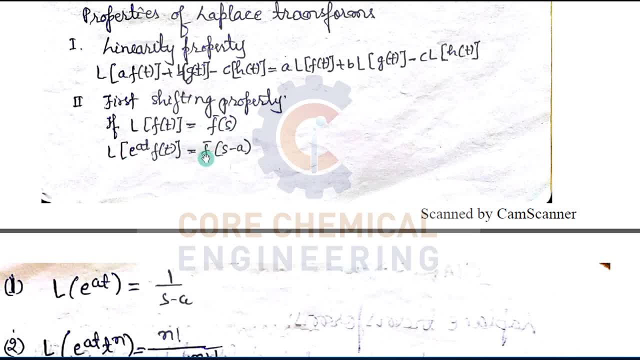 then l of e at f of t is equal to will, is equal to f, s minus a. suppose if you are knowing that any function, okay, f of t, uh, has a like a laplace transform of this function, and now you have to calculate l of e of 80 f of t, then what you can do instead of s, what you have calculated in the 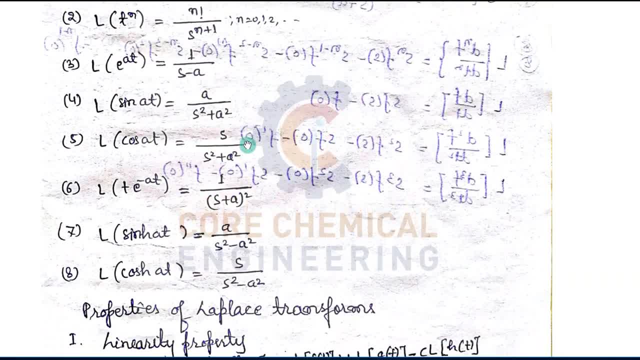 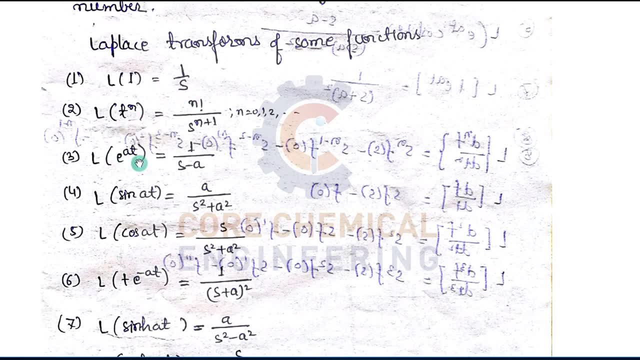 function. you just put s minus a like: uh, i'll show you here somewhere. suppose this one, what you have done: l of 1, b, no. 1 divided by s. okay, then l of e at raised to power, e at is equal to what will happen. 1 divided by s instead of s, just pushed. 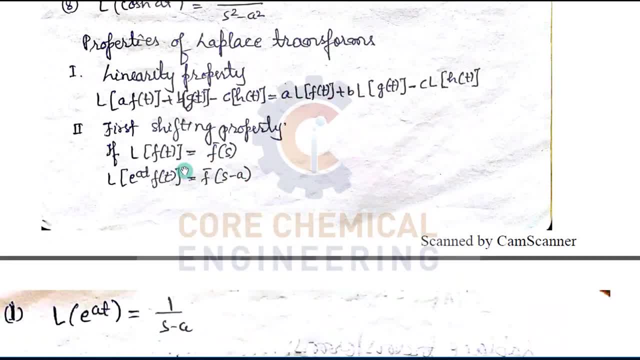 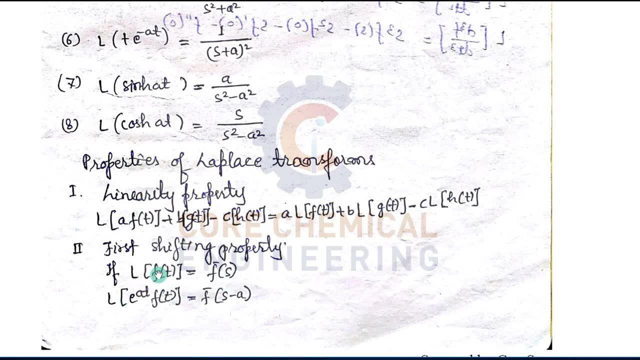 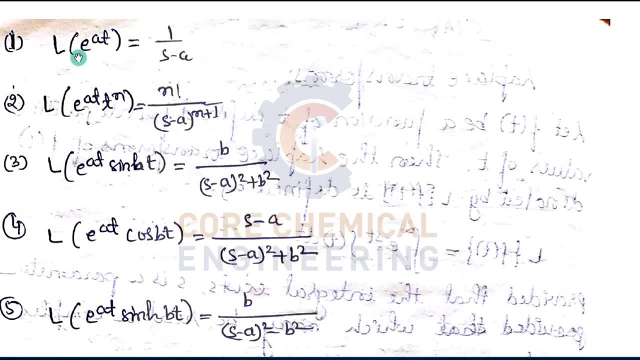 s minus a, 1 divided by s minus a. so like that you can use in any uh laplace transform function. this, like this formula, you can use in uh, this kind of laplace transform function, uh. now examples. these are the examples. examples for that. you can see it here: l of e at what you have told you. like l of e. 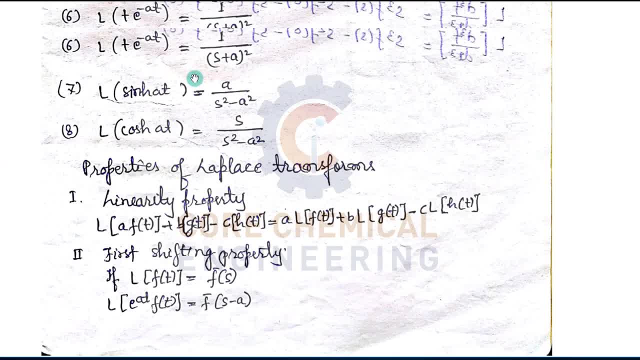 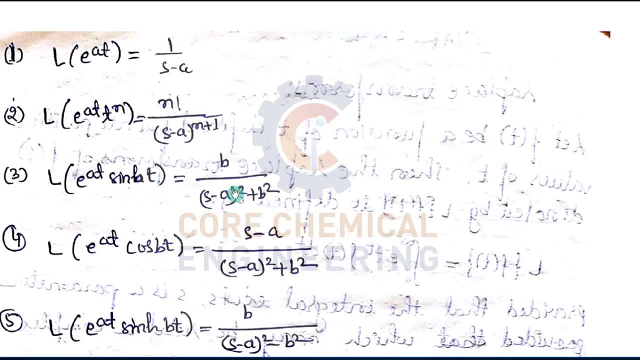 80 t raised to power and in fact you are divided by s minus a n plus one. you see it here, okay: s minus n plus one. like that e of a t sine b t, then b divided by initially is to be s, s square plus b square. now you have to put instead of s, 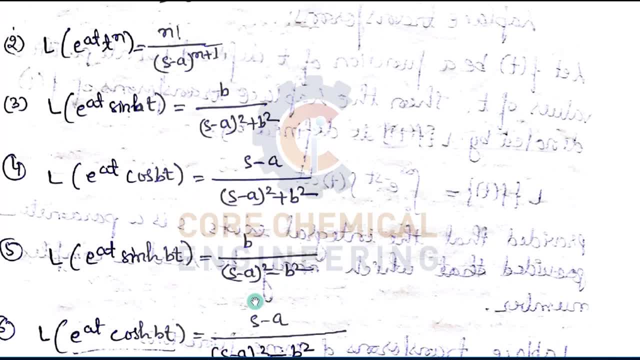 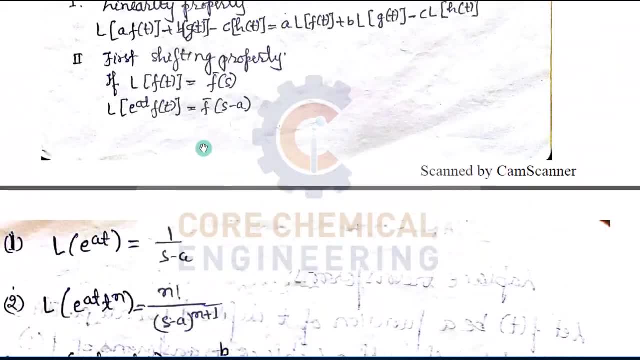 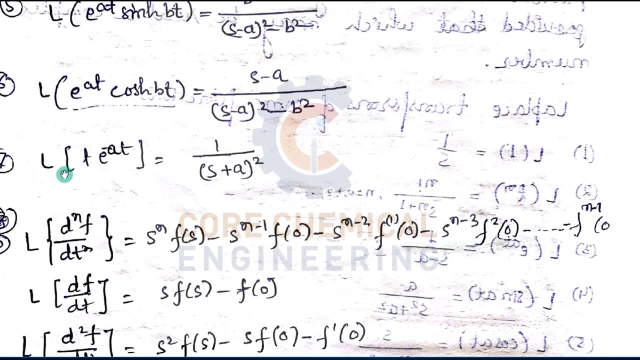 s minus a square, like that. these are the formulas that you can write it down. if you remember this, you don't don't remember this formula, just remember this property, right? so this is the very important property that you must remember now. l of t into e, d, e raised to the minus of 18, so here minus it is there. then what? 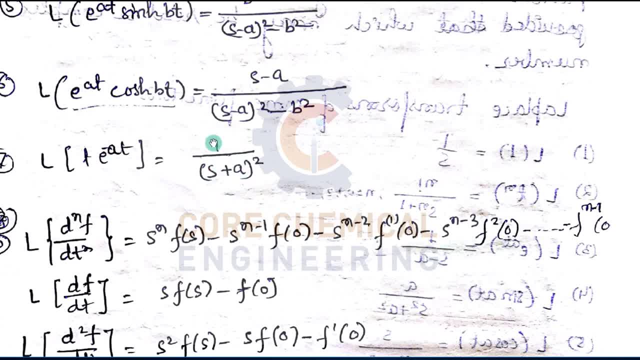 happens s minus of minus a, so it will become s plus a. so initially l of t. what? what would be the l of t 1 upon s square? then l of t into e, raised to power minus 80, will become, will become equal to s plus a whole. 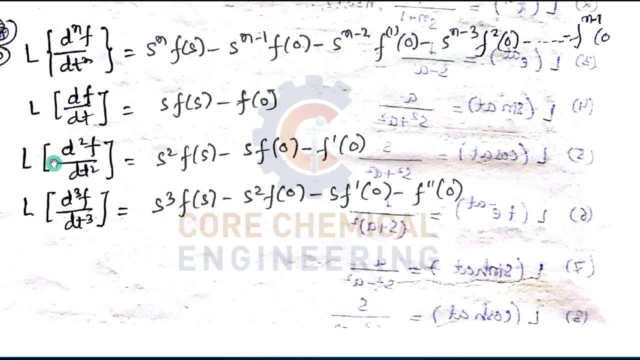 square right now. this one is very important. this is the thing that we are going to use repeatedly in the process dynamics and control system, right? so if you want to calculate the- you know- laplace transform of any differential function, suppose of order n, l, the laplace. 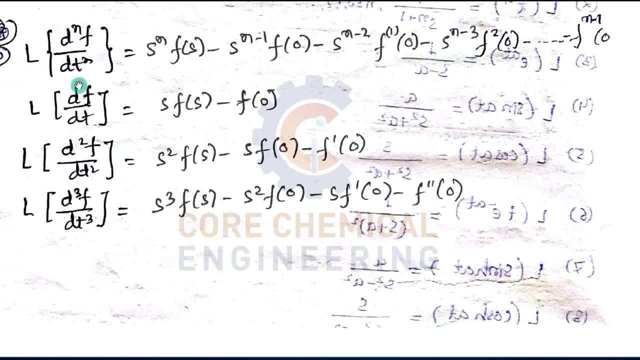 transform of d raised to power, n, f divided by dt, and so any function with uh having order n. okay, so for another order, laplace transform. this is how you can calculate the laplace transform. you can write it in this way, now, suppose like that, only if you want to calculate the for the first. 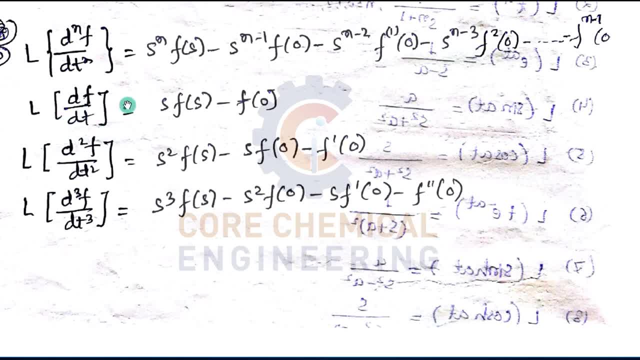 order system l of df by dt. okay, so what will happen? you say one, all right, instead of one. you just start: instead of n, you just write one. so yes, f of s minus. you just put one here. so what will happen? one minus one, zero. so s of zero is equal to one. 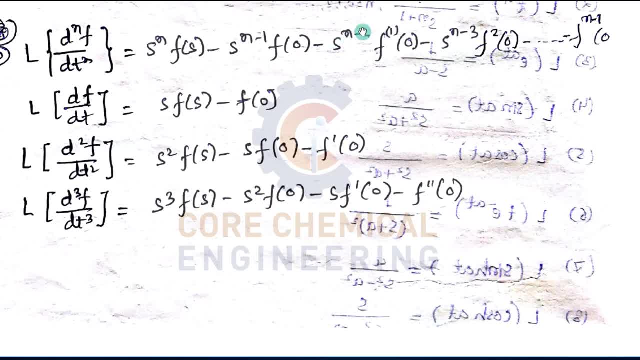 here: f of zero minus s of one minus two. so once it start going into the you know negative value, you don't, we don't, we don't need to take this, okay, so this much only we require now. similarly, l of d square, f divided by dt square is equal to: just put n is equal to two s square here: f of s. 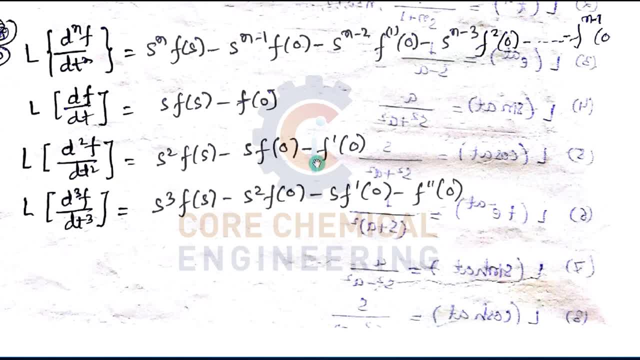 minus two. just put here two s into f of zero minus, here n two s minus two. so this is the n two minus two zero. so here s raised to power, zero becomes one. here f dash zero. so this is how you can calculate, calculate the laplace transform of any differential function. this is for first. 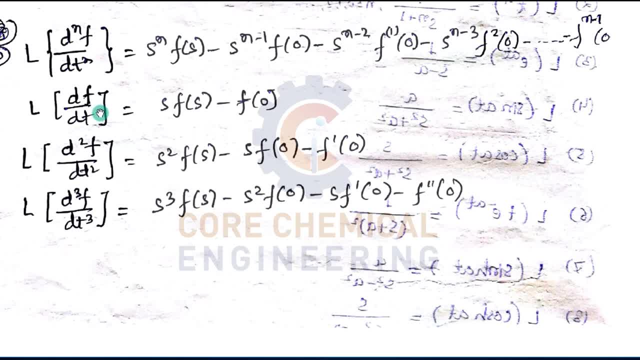 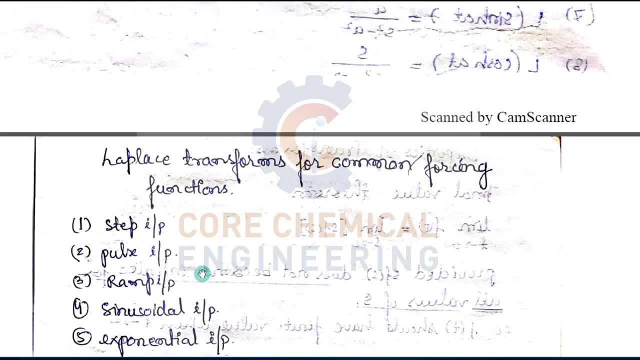 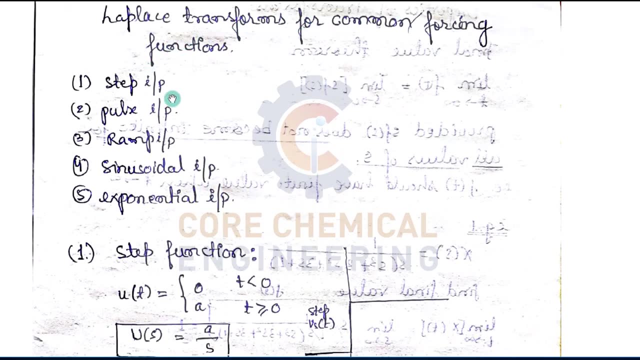 zero order, first order. this, sorry, this is for first order. this second order, this is for third third order. so you must remember all these formulas. now, in this chapter only, we will continue to study laplace, transform, common forcing function. so so suppose a function has been given. these are the kind of input, like you know, in in the process. 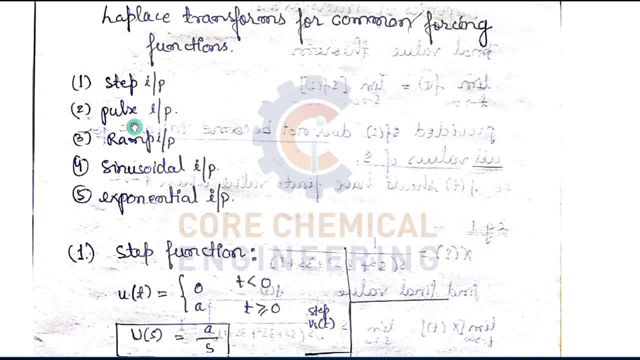 dynamics and control. these are the like a input that we inject. so we must know the laplace transform of this function. suppose the step input is there, so we know the step input function, we will be knowing. so what will be the laplace transform of that then? pulse input, ramp input, sinus order input. 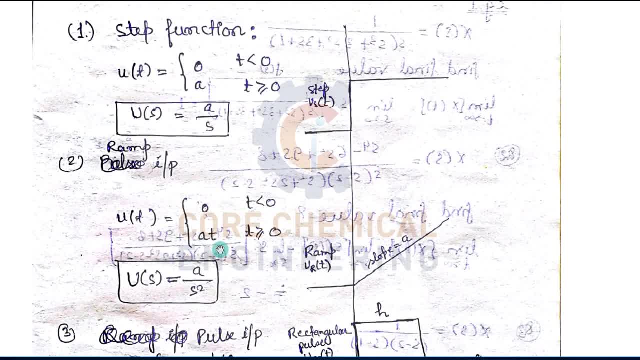 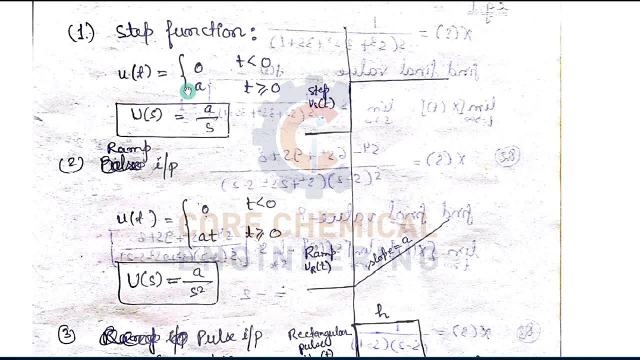 exponential input. all those things will discuss. suppose here comes the step input. the step input make your theory: u of t is equal to zero when t is less than zero and u of t, your u of t, becomes a when t is greater than or equal to zero. so what happens similarly one time if 0 remains? so what happens following that function? 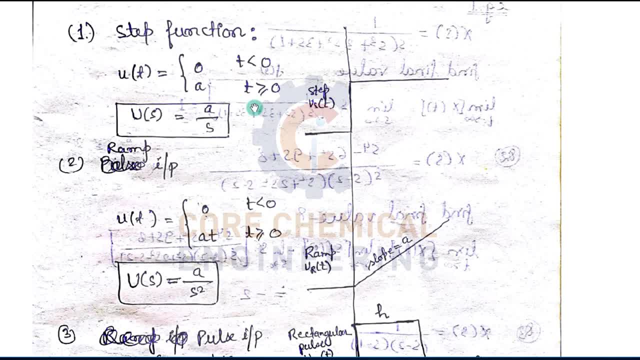 the outcome happens is that you have a 0. suddenly, as you have a t is equal to or greater than 0, it suddenly increases its value, and after that it will go constantly. so that is why it is represented in this way. so what will be its? u of s is equal to, because its is zero. so what will become a by s right? 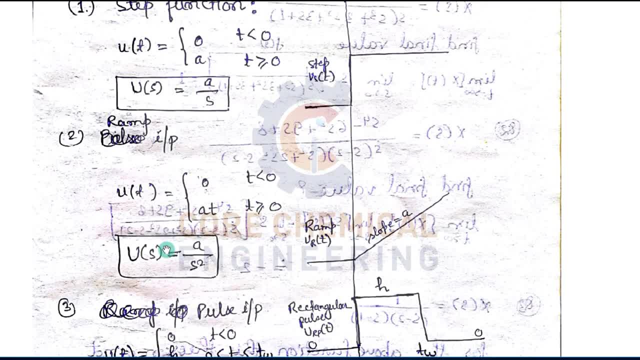 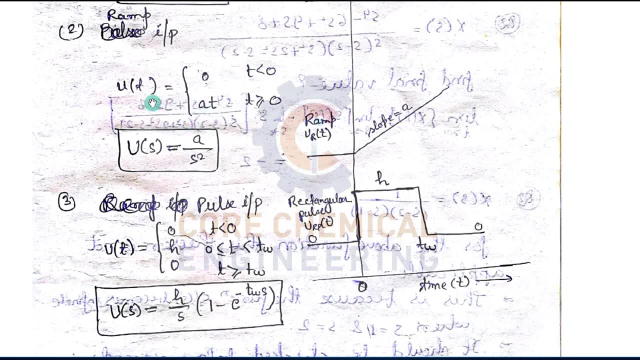 because its is zero. so what will become a by s right? so that is why u of s is represented as a by a. similarly, for ramp input, u of t is equal to 0,. 1t is less than 0, u of t is equal to 80,. 1t is greater than or equal to 0. 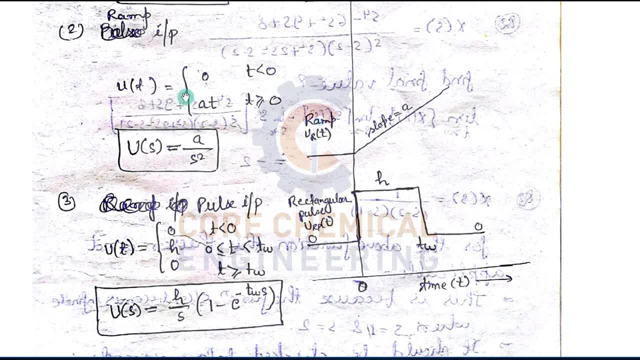 so this is linearly vary with the kind of y is equal to mx. this would be the slope for that. so here you can see it, when your time will be 0 or less than that. so what will happen, like this time will start to go in positive. 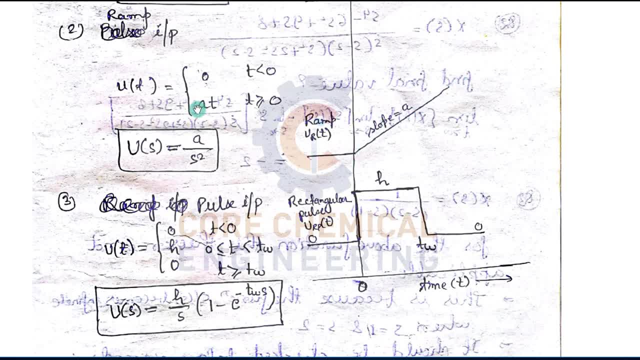 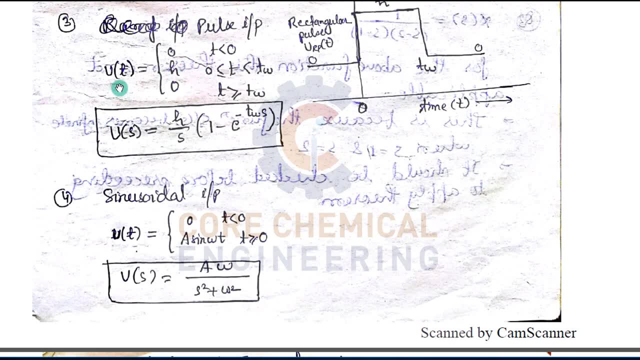 it will vary in straight line. so if you take out the last transform of this, u of s is equal to a divided by s square. similarly, for pulse input, u of t is equal to less than now. what is u of t? t is less than 0, so value is 0. 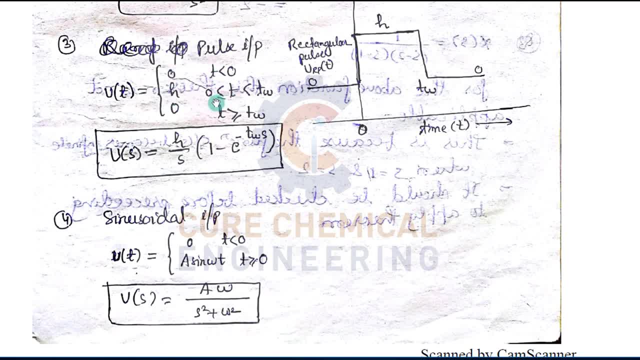 when pulse input is when your time is between 0 to t, when your time is between 0 to tw, so its value is h. like after tw your time travels, its output is 0. so means in pulse input what will happen? like your time is less than 0. 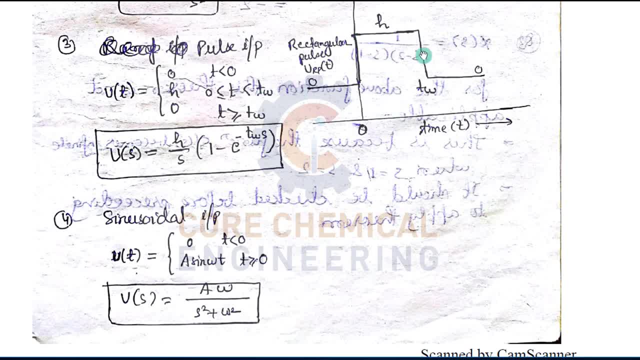 so its value will be 0. certain time period means some time period. t, ok, from here to here. in that time period, its little bit means your outcome will come, output will come. so what is its value? h will come in that duration under. after that, what will happen? 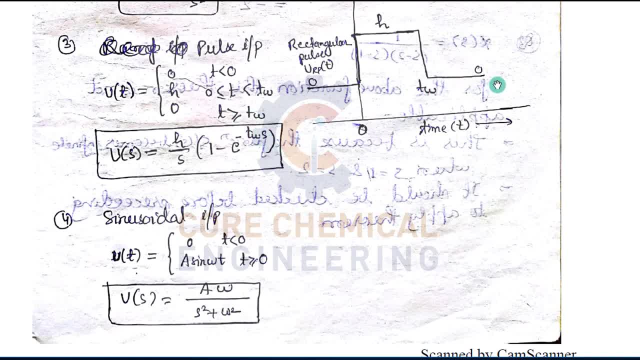 that as you cross tw time, its value will be 0 again. so this is pulse input. means for certain duration of time, for very short duration of time, for tw, we give an input. so this is pulse input. now sinusoidal input. what is sinusoidal? that will vary, like. 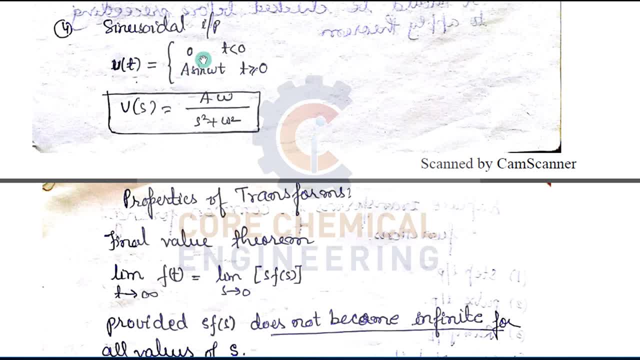 vary like a sine and cosine. so here you can see: u of t is equal to 0 when t is less than 0. when u of t is equal to a sine, omega t when t is greater than or equal to 0. so if you take the laplace transform of this, 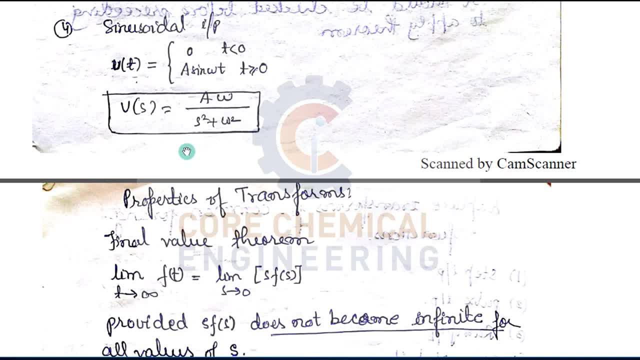 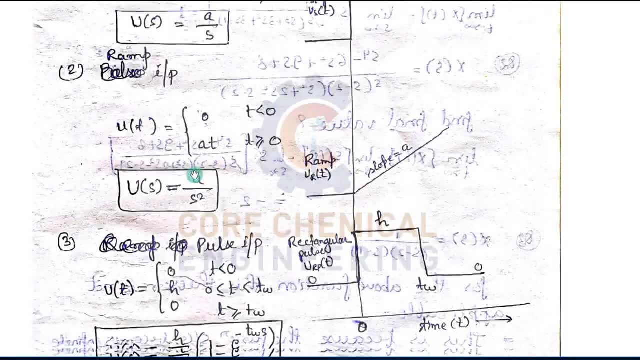 you know, there is laplace transform of sine function: a into w divided by s square plus a w square. ok, so this is, these are the common forcing function that you must remember. ok, now, in this tutorial, only, in the continuation of that only, we will study here only. 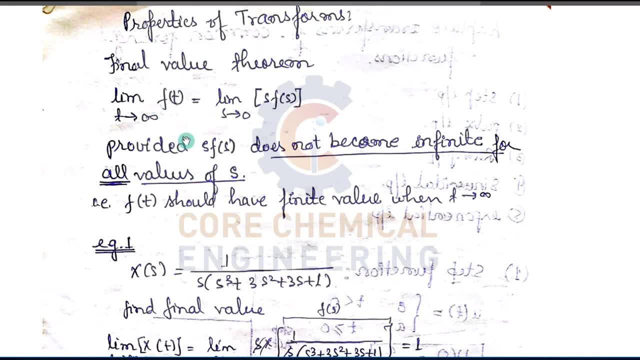 properties of transforms. so here we will discuss two things: final value theorem and the initial value theorem. you must remember the concept of final value theorem and initial value theorem and the examples based on that, because to i had seen that two to three times in the gate exam. 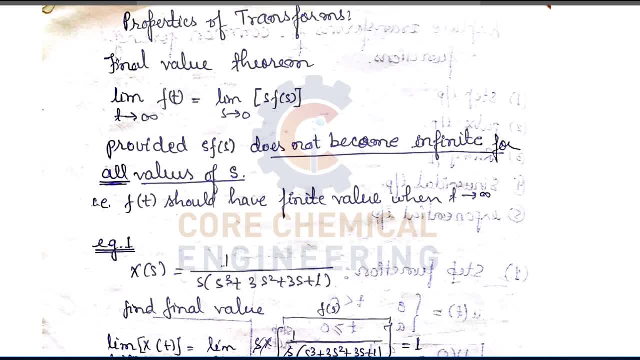 they had asked the question based on the initial and final value theorem. so what does final value theorem says when a t, when a limit, suppose any function f of t is there. now, if we want, we want, we want to know about the final value, what would be the final value? 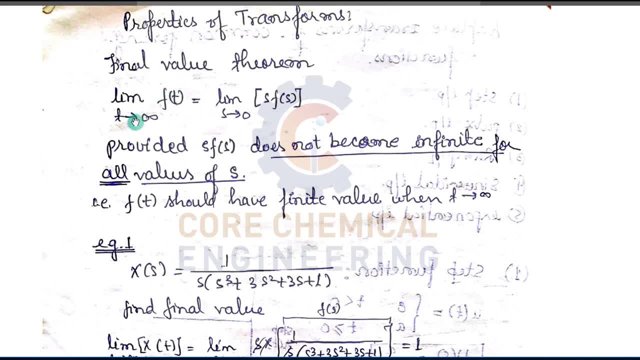 with respect to the time. suppose your time, any function. we have given f of t, and if we take times as infinity means infinitely time after infinite time, what would be the outcome of that? ok for that. so so limit t tends to infinity. f of t value what will come? 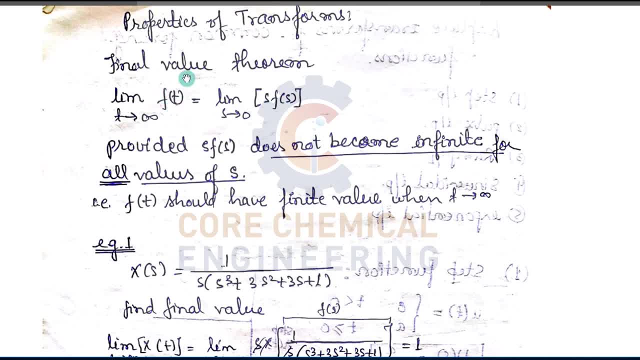 is the limit of s into f of s. we have to calculate the f of s of f of t, curve, Laplace, transform, linear, just put it here. then just put one more more s in multiplication of f of s, then put s tends to zero, so limit s tends to zero. 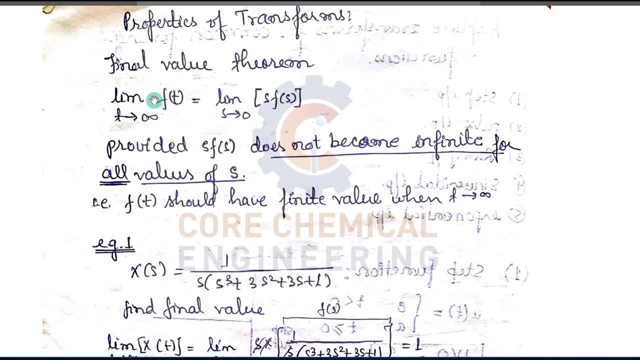 s of f of s will. if we put like this, we will get the final value of f of t. ok, so provided s of s does not become infinite for all values of s. so you must remember this when you are going to put the value of s. 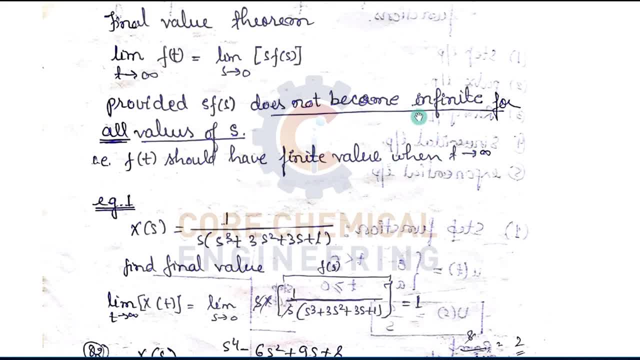 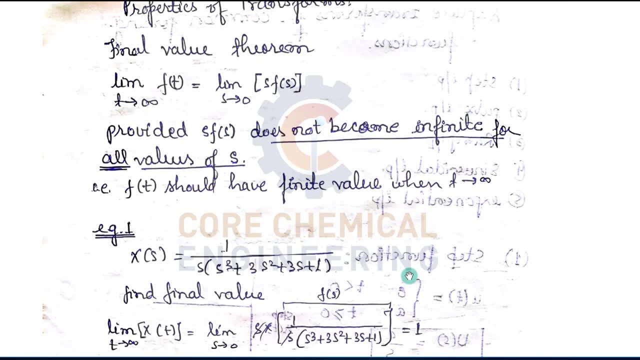 ok, so f of t should have a finite value when t tends to infinity. and one more thing: f of t must have a finite value when we are going to put t tends to infinity. now example: you can see it here. example: given one, now function: given x of s, 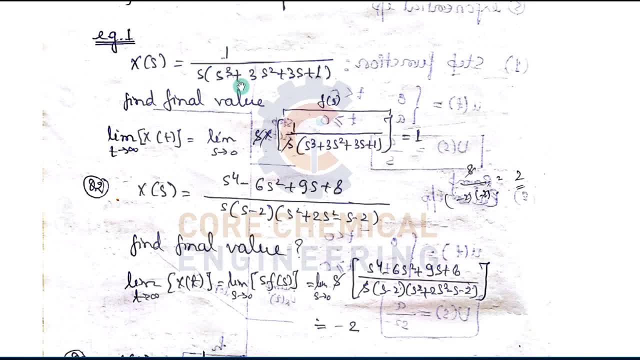 directly. here. it is given 1 divided by s into s- cube plus 3s square, plus 3s plus 1. ok, now we want to calculate the final value of this. so what will happen? just push limit. t tends to infinity. x of t is equal to. 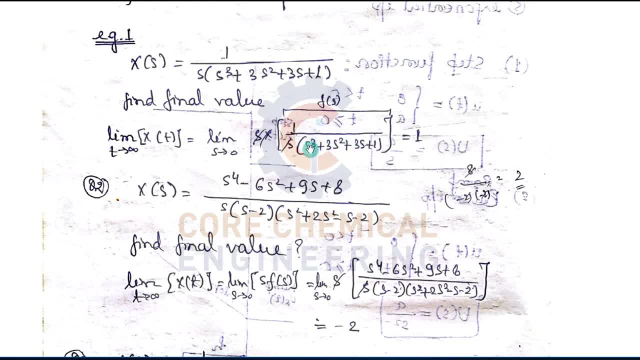 limit s tends to infinity s into this function. just push this function s will cancel. you put 0, 0, 0 here. we will get 1. so this is the final value. similarly, question 2: this is your x of s. now we want to calculate. 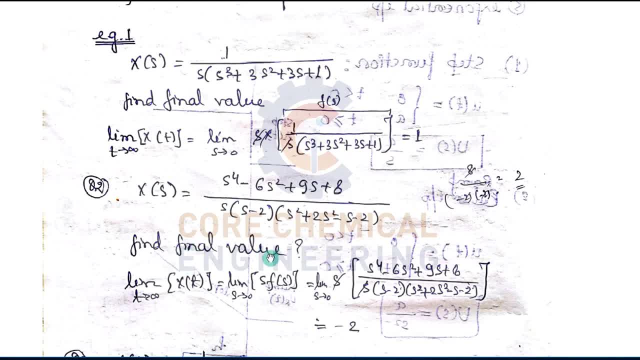 the final value of this, then limit of t tends to infinity x of t, then limit of s tends to tends to 0, s into f of s. ok, so it will get cancelled. now put s equal to 0 here, everywhere. so put s equal to 0. 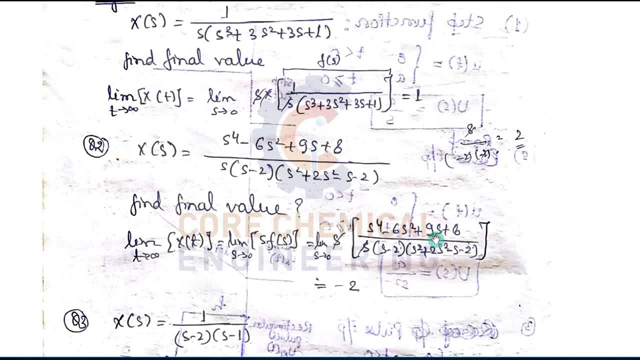 here everywhere. if you put s equal to 0 everywhere, you will get the value 0, 0, 0 here. 0, 8 divided by minus 2, into minus 2, into minus 2, 4 divided by. so you will get the value 2, not minus 2, ok. 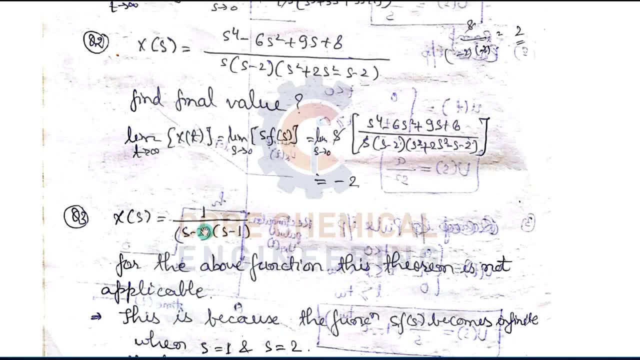 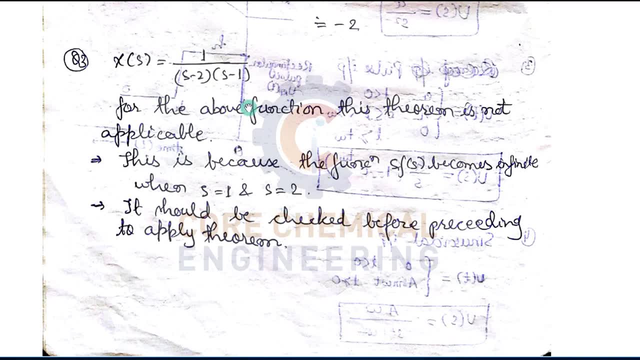 for the above function. this theorem is not applicable. x of s divided by s minus 2 into s minus 1. because this is because the function, because when you put s equal to 1 or s equal to 2, here, if you put s equal to 1. 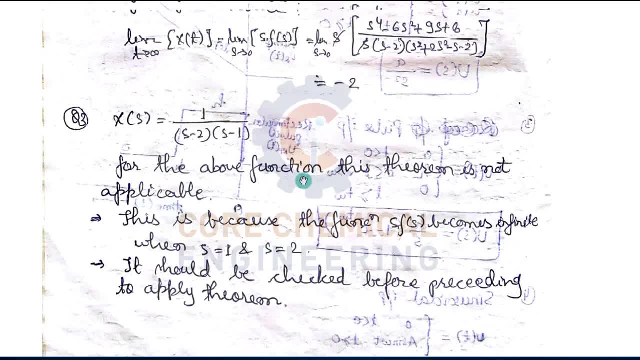 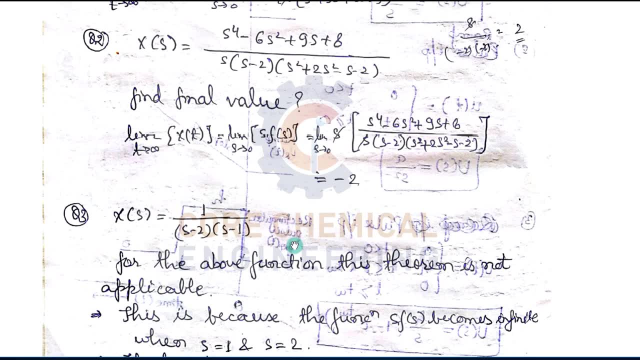 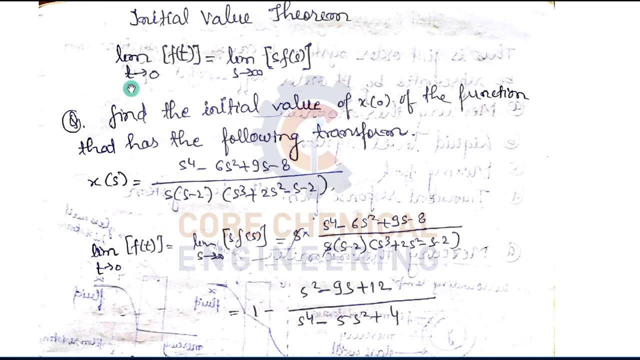 it will be infinite, so it should be checked before proceeding to apply theorem. ok, so if you are going to put the value initially, you must check, like ok, whether it is going to become infinite or not. now, initial value theorem will limit t tends to 0. f of t. 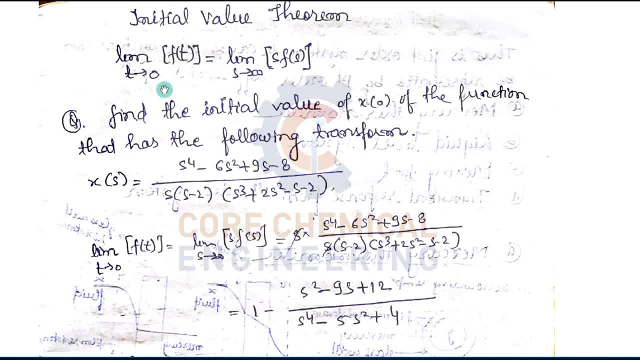 dt if you want to get the stand value, initial value when you are going to give a time. t is equal to 0. if we have the function f of t, then what we will do, we have to do, we have to take limit s tends to infinity. 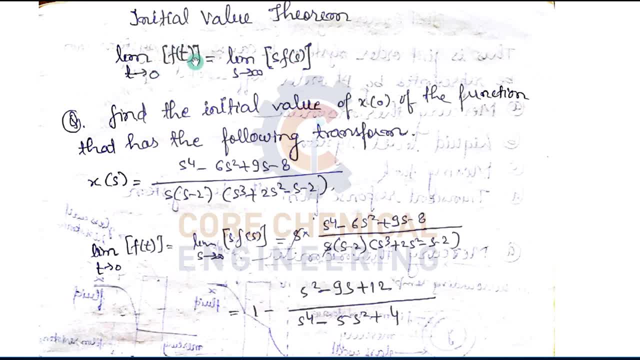 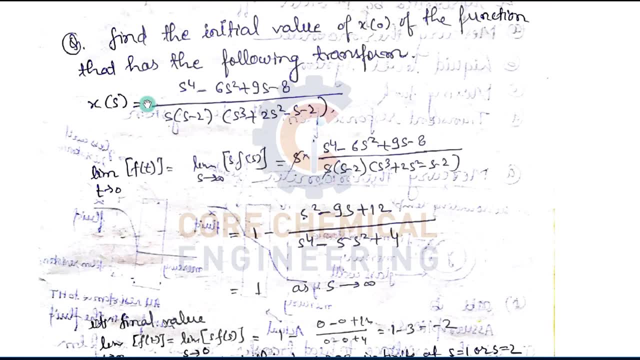 multiply s into f of s. f of s is the laplace transform of f of t. ok, so in that in this kind of question we can solve by using this formula now. now, here you can see: find the initial value of x of 0 of the function. 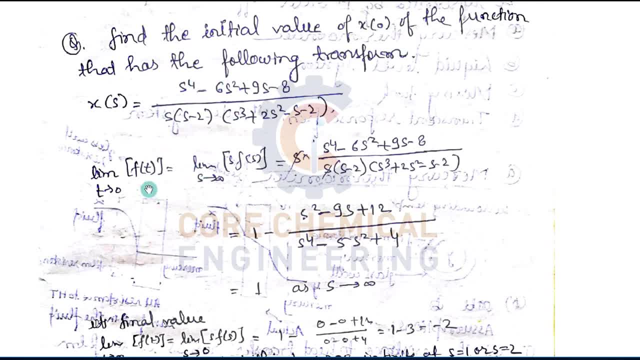 that has the following function: x of s. given this function, now we have to calculate the initial value. so in the case of initial value, what we do- limit t tends to t tends to infinity. f of t is equal to limit s tends to infinity. s into f of s, so s we just multiply s into the. 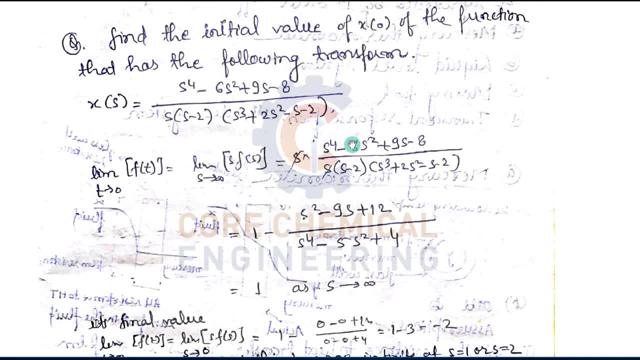 whole function and tells: put s tends to infinity, we'll, we'll get after after you this whole term we can be. we can represent in this form: 1 minus s square minus 9 s plus 12, divided by s raised to power, 4 minus 5 s square plus 4. now, put s raised to power s tends to infinity. so this: 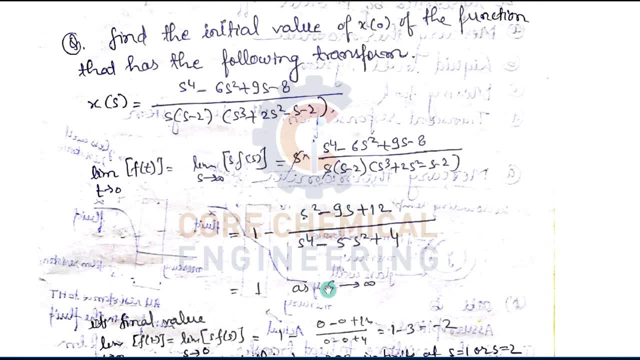 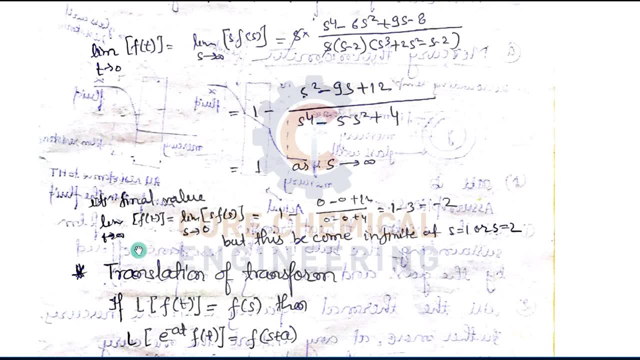 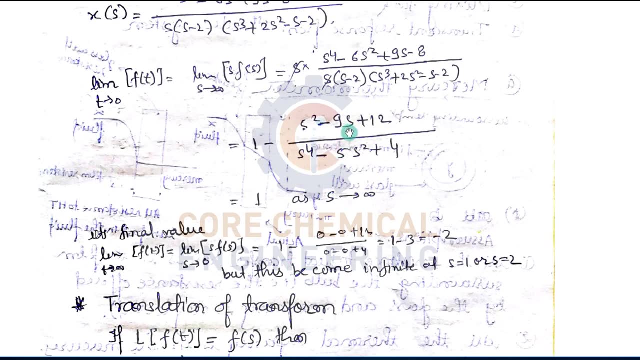 becomes some, we'll get some value and divided by the infinity, we'll get the value of 0. so we'll get the initial value as 1. but if you want to calculate the final value and what happens, t tends to infinity. f of t is equal to limit. s tends to 0, s of f s 1 minus. now just put s equal to 0. 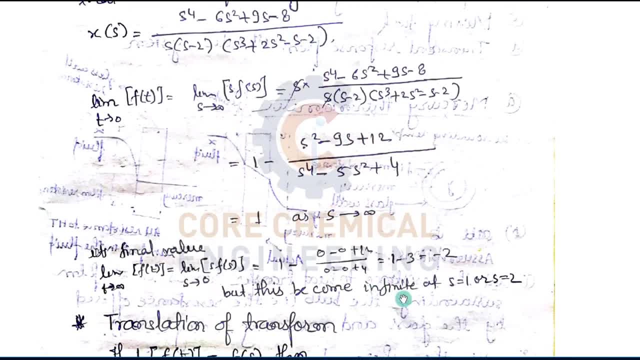 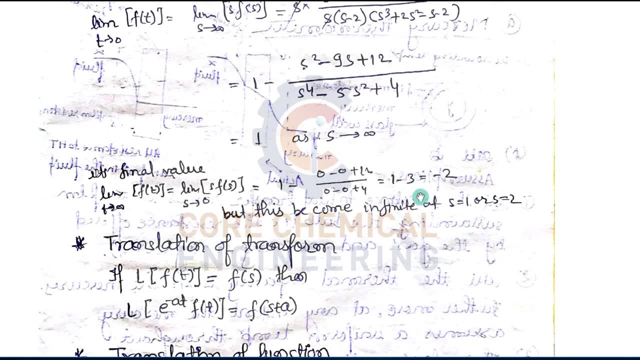 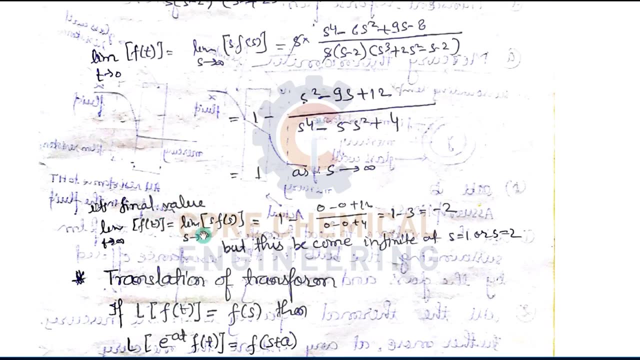 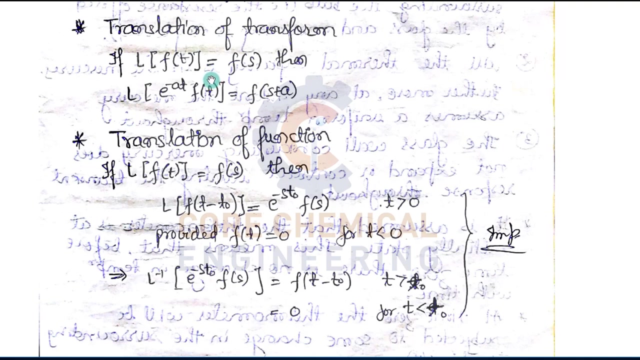 so we'll get minus 2. but what happens here? if you put the value s equal to 1 or s equal to 2, here it becomes the infinite right. so we cannot basically use this formula for getting the infinite value. you, you, you, you- final value from this formula. right now let's discuss lap trans, some other you know, important. 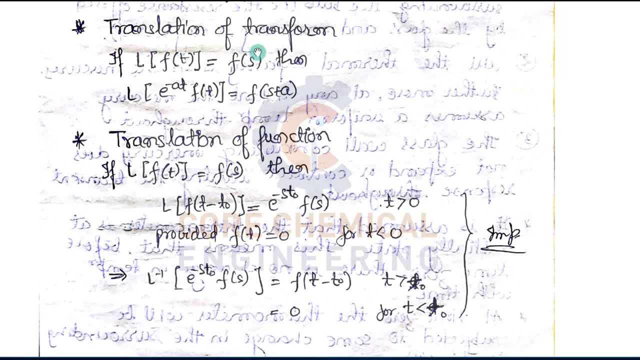 formulas with respect to the laplace transform. so another is translation of transform. so if l of f of t is equal to f of s, then just remember, l of e raised to power minus at f of t is equal to f, f of s plus a. now translation of function. so if l of f, t is equal to f of s, then l of f. 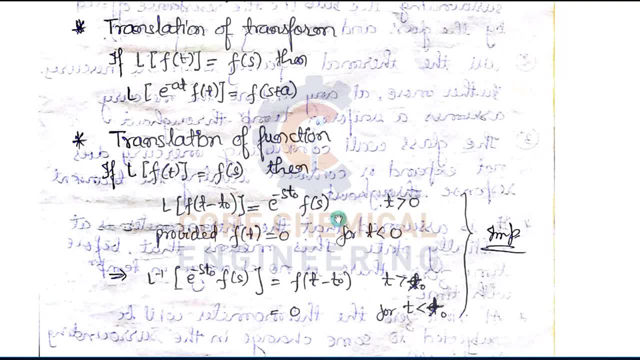 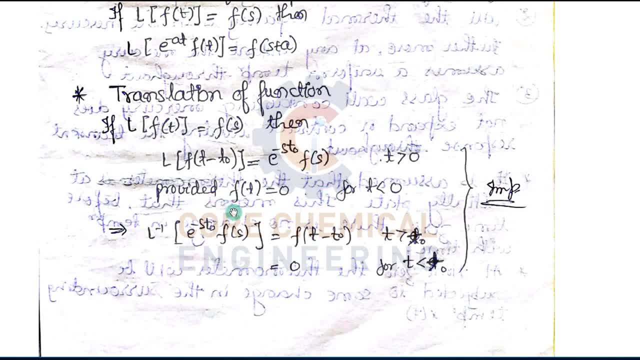